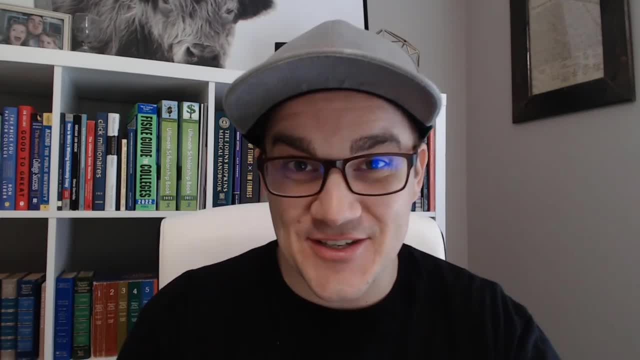 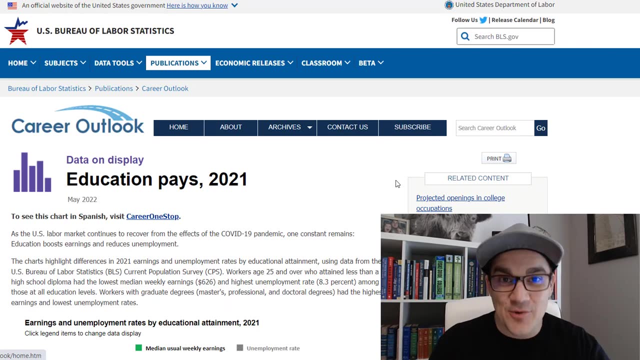 straightforward numbers. They're going to show you how much money you should expect to earn by education level. As you can see here we're visiting the US Bureau of Labor Statistics. The reason why I'm here is because I'm going to show you how much money you should expect to earn. 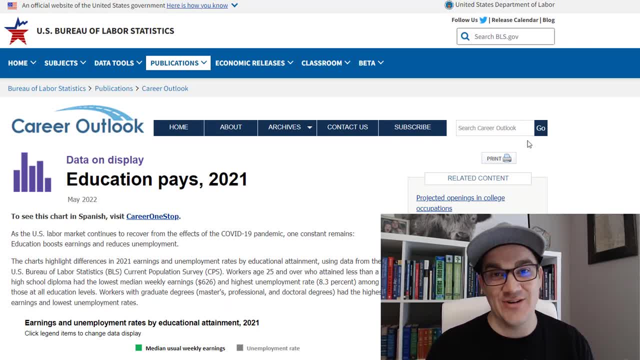 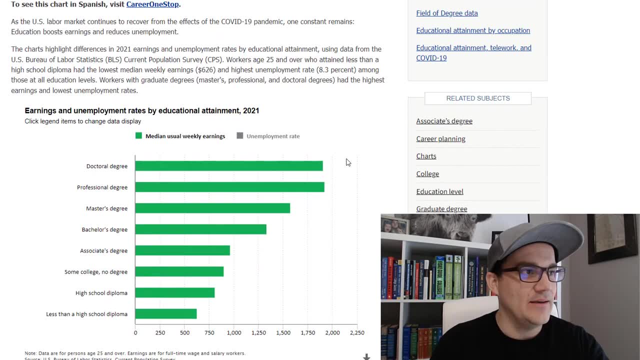 by education level. The reason we're here is because this is really really accurate data. okay, So the trend that like, hey, you don't need a college degree to make good money, let's actually compare real data. okay, As you can see here the higher up on this chart, 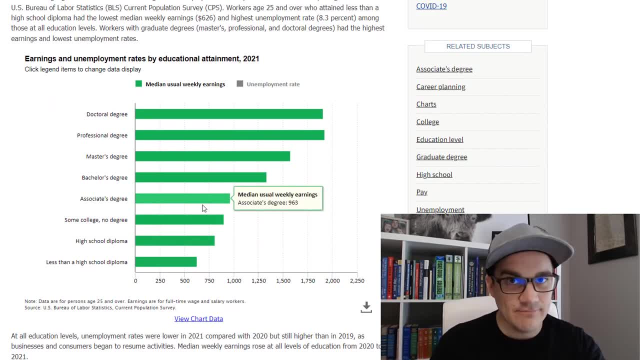 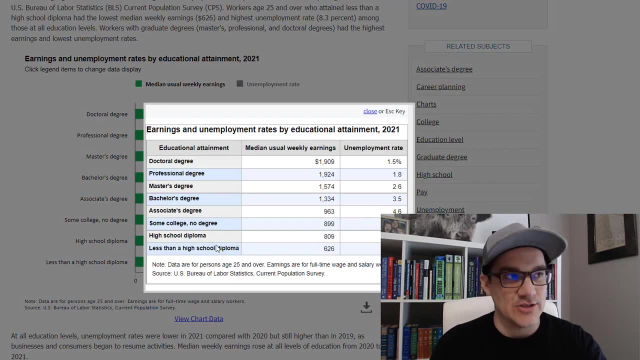 the higher up your education level, the more money you make. That's pretty straightforward. We probably all knew that, but let's break it down by numbers. okay, We're going to view the actual numbers. If you have a high school diploma every week, your weekly earnings: 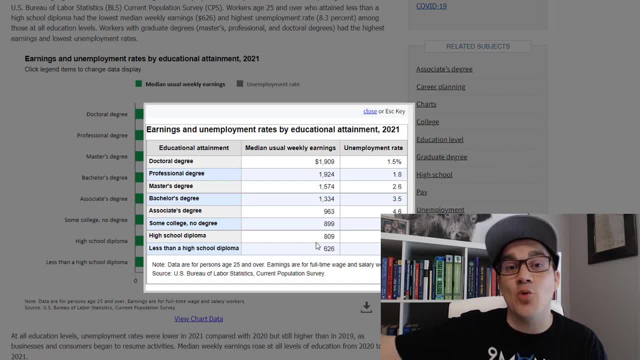 should be about $809 per week. You might make more than that. If you do make more than that and you go get a bachelor's degree, you should expect to make more than the average bachelor's degree earnings as well, but this is average. okay, Now, if you went to college but dropped, 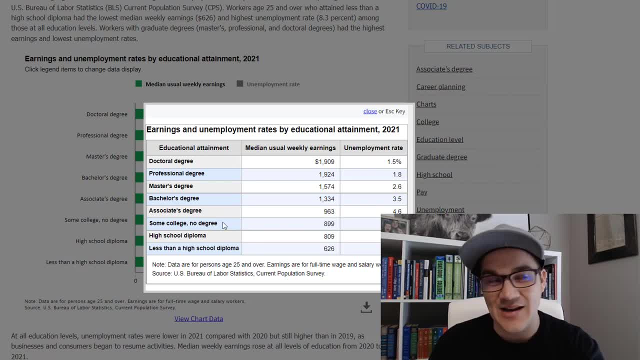 out of college, the average weekly earnings is $899.. Associate's degree: $963, and if you notice here, from a college dropout to having an associate's degree, it's, I mean, $64 a week in difference. If you went to college but dropped out of college, the average weekly earnings is $899. 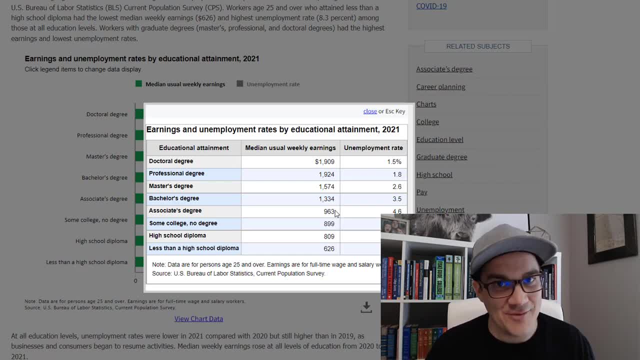 In like increased earnings. that's really not very much so. that's interesting to point out. Now, a bachelor's degree: if you have a bachelor's degree on average, you're going to earn $1,334 per week. Master's degree: $1,574,. all the way up through a doctorate degree: $1,909.. Now 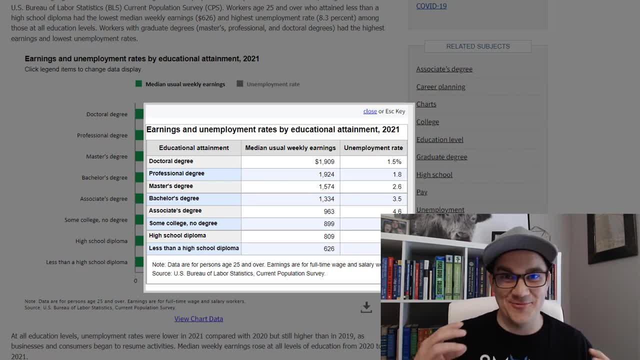 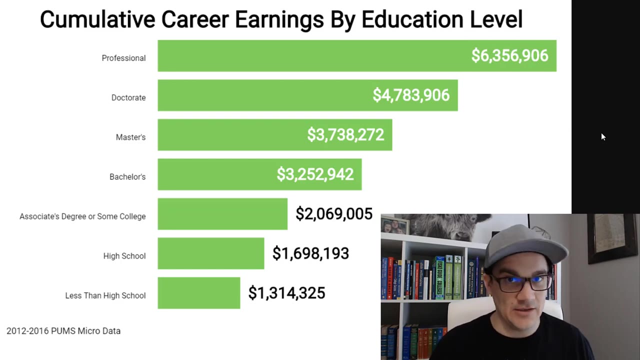 I know that weekly earnings it's kind of hard to like kind of lay the big picture out and calculate how much more you're going to earn by the end of your career. so I want to jump over to another graphic That breaks down career earnings based off of income level or education level. okay Now. 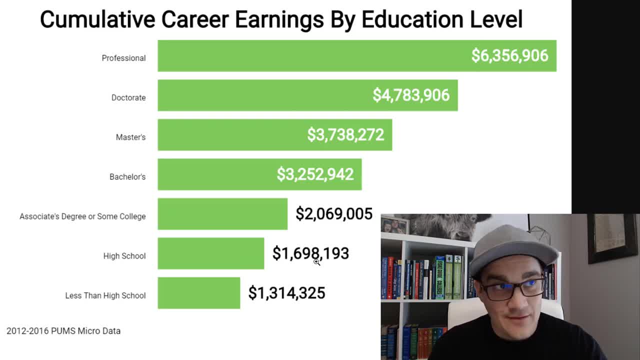 as you can see here, a high school grad will make almost $1.7 million by the end of their career. If you have an associate's degree, that's going to jump up by just over $300,000 by the end of your career and be just over $2 million in career earnings. okay, So that's going to be. 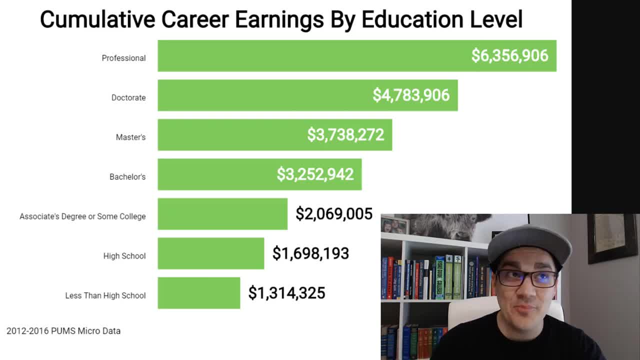 in your entire career. Now the big jump is when you actually go and get a bachelor's degree: $3.25 million in career earnings by the end of your career. So that's a huge jump. That's like a million and a half- more than a million and a half dollars more if you have a bachelor's degree. 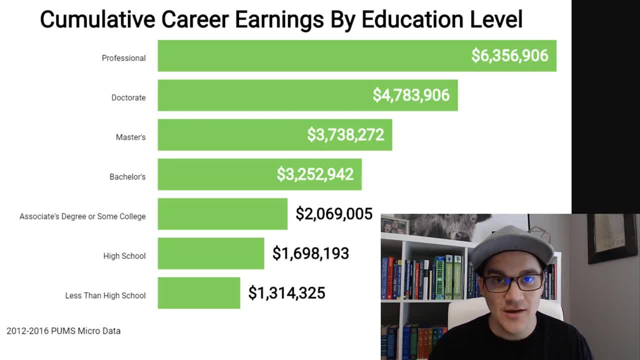 versus just a high school diploma. okay, Now, what would be different in your life if you made an extra million and a half dollars in your entire career? That's a huge jump. That's a huge jump: $2 million. by the end of your career, You're going to live in a different house. You're going 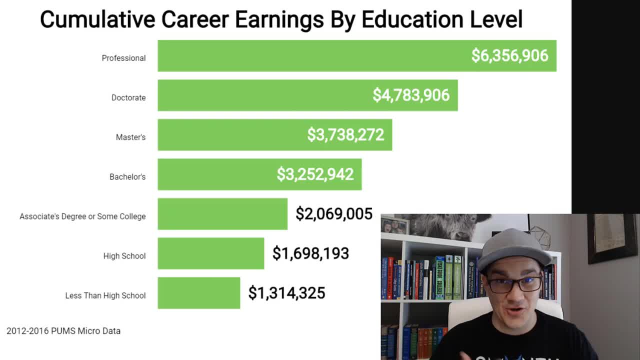 to drive different cars, Your kids might go to college much, much easier. As you can see, master's degree is going to add an extra about $500,000 to your career from bachelor's to master's degree And, as you can see, a professional degree, over $6 million by the end of your career. 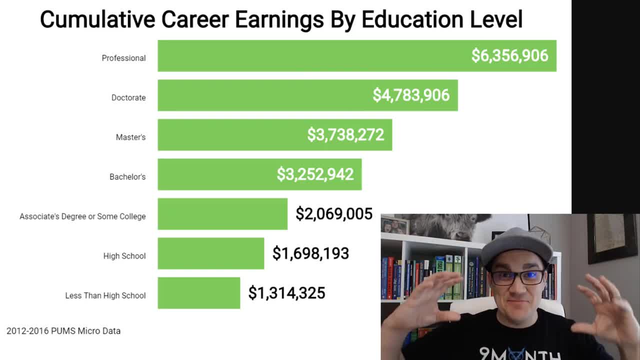 So there are some big jumps. It gets bigger and bigger the longer time you calculate and the more education you have. okay, This is straightforward. We've all known our whole lives that if you go get a college degree, you qualify for better jobs. 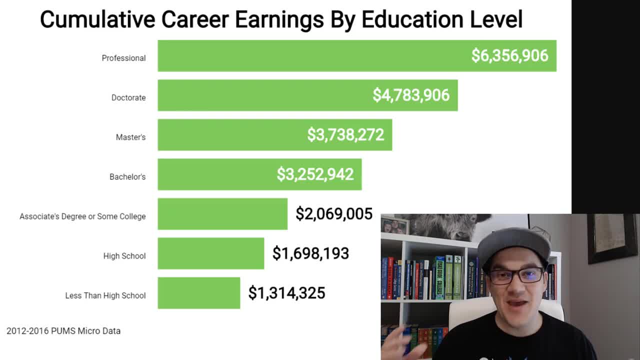 you get pay raises. But there's this huge trend on the internet basically saying you don't need a college degree anymore. Well, the numbers show that's completely false. Yes, you can succeed without a college degree. You can, But the majority don't. The majority people. 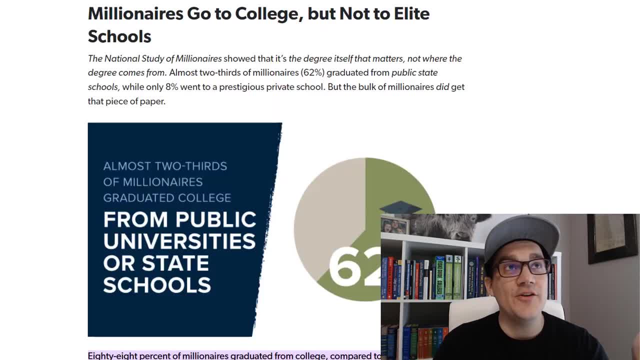 with college degrees, don't? They don't have a college degree. They don't have a college degree. Make more money Now there's one other thing I want to show you here, And this is a study called the National Study of Millionaires by Dave Ramsey. I don't know if you've heard of Dave Ramsey. 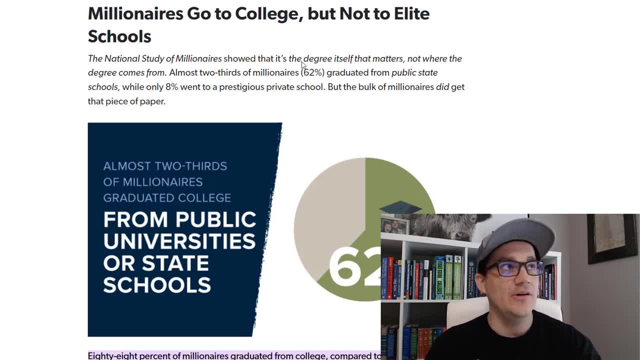 but he's a financial guru, okay. Now, as you can see here, he says further up in this article, and I'll leave a link in the description: but 80% of millionaires have college degrees, okay. 90% of billionaires have college degrees, okay. 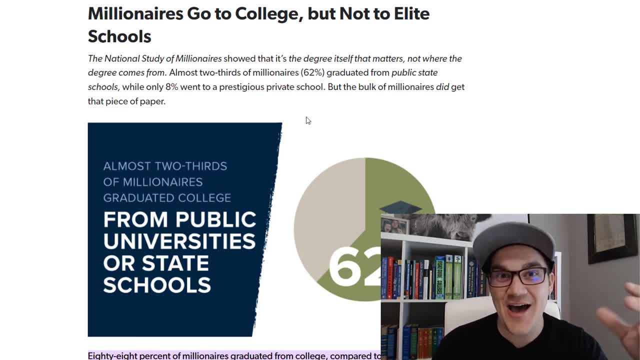 But, as you can see here, where you go to school does not matter if you're actually calculating millionaires and college degrees. 62% of millionaires have degrees from public universities or state schools, So not the Ivy League and stuff like that. okay, The important thing is actually: 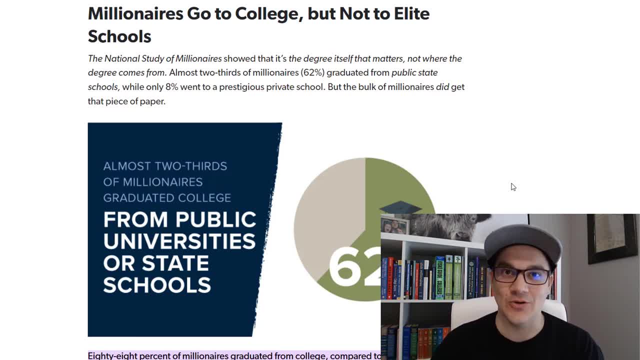 getting the degree not where you actually went to school. okay, And yes, if you want to go work at a law firm in downtown New York City, maybe you need to go to Harvard or Harvard University, Harvard or Yale or something like that. okay, But for the most part, to have a successful career, 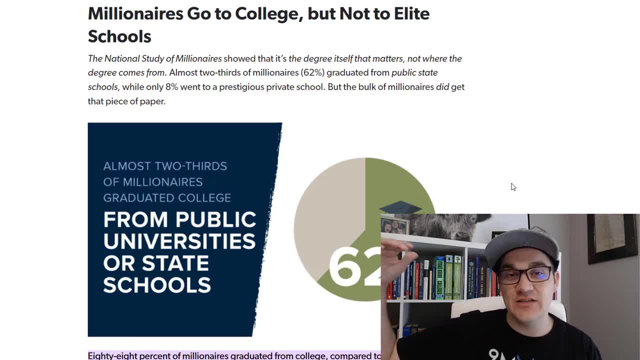 college degrees make a huge difference. Ivy League degrees, I mean, they're good for specific jobs if you have a specific need for it. If you don't have a need for it, I mean: look at this, It's pretty clear. okay, Now the big challenge with getting a college degree is that it takes 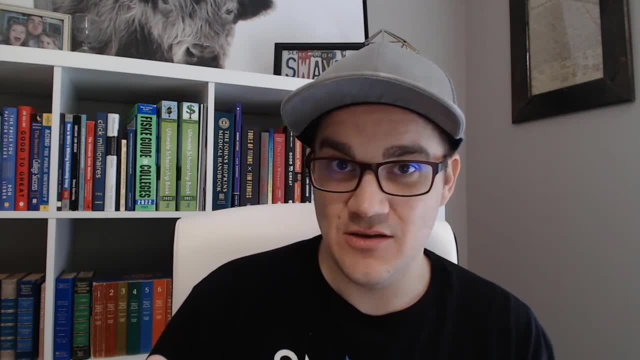 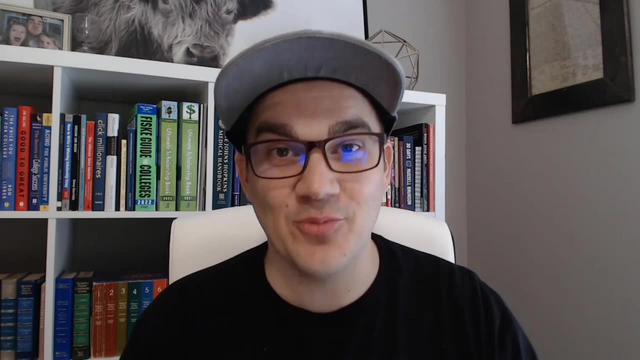 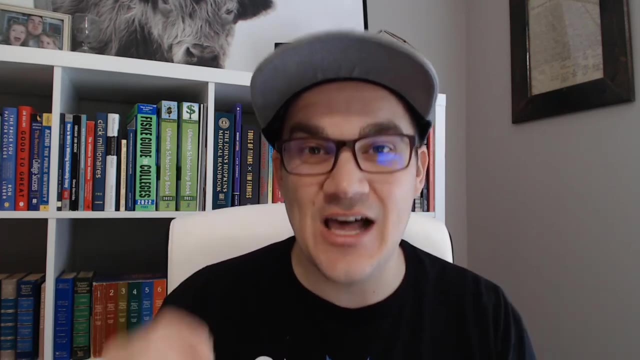 on average, about six years to get a bachelor's degree and, on average, costs about $90,000.. Well, colleges are pushing online programs because of the pandemic, and online programs are faster and easier if colleges let you accelerate at your own pace instead of going at their pace. okay. 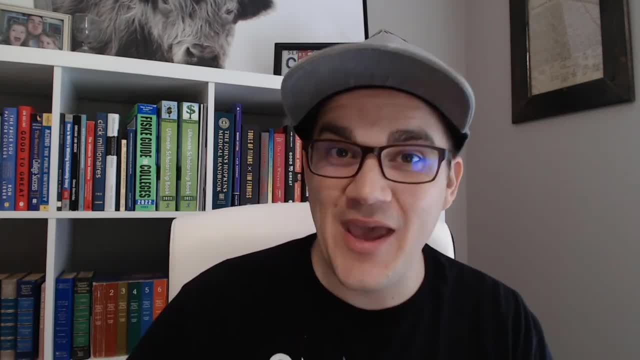 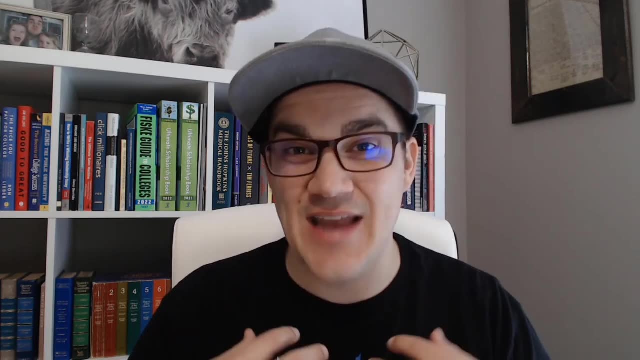 So if you find, basically, a college that offers a self-paced program, you can accelerate really, really quickly and earn an entire bachelor's degree in less than a year. I personally did it in nine months and when you're talking tuition it's like less than $10,000.. 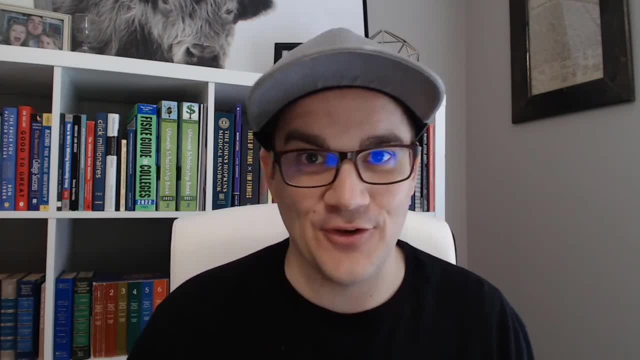 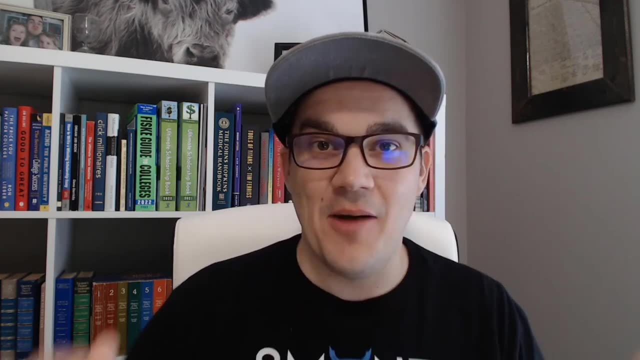 Down to as little as basically free if you get scholarships and grants. okay, If you're interested in getting a college degree really fast, accelerating your degree, I'm going to leave a link down below to another video that's basically a full-blown tutorial on how to hack. 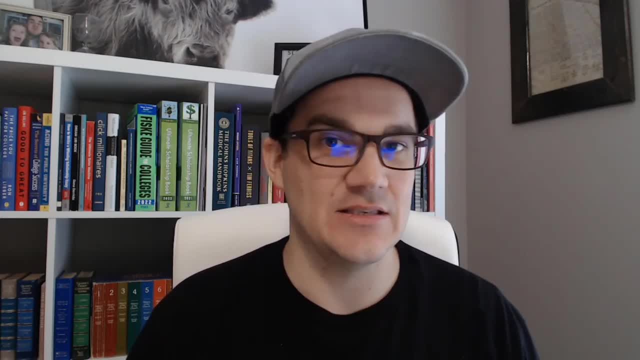 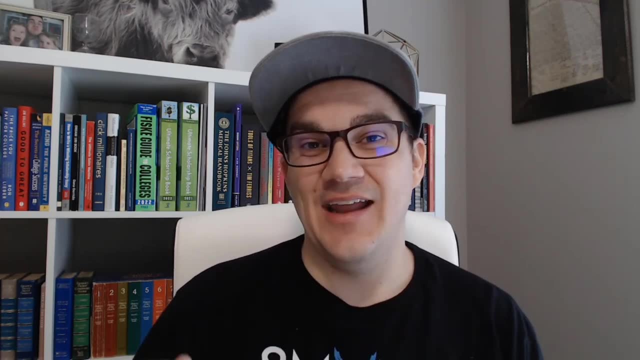 college and earn your entire bachelor's degree in less than one year for literally pennies on the dollar. I'll leave that link down below. I hope this video has added value to your day and helps you calculate how much more money you'll make with a degree.